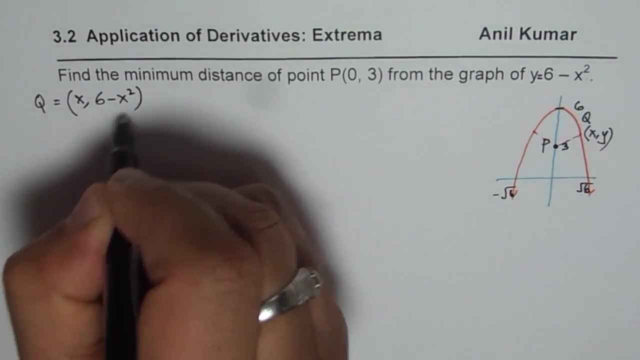 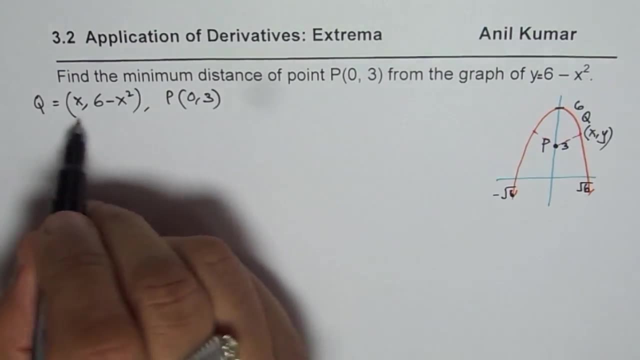 So if I say point is x minus x squared, is that okay? 6 minus x squared will be my y coordinate And we have a point P, which is 0, 3.. The idea is to find the distance between P and q, So we can use the distance formula. 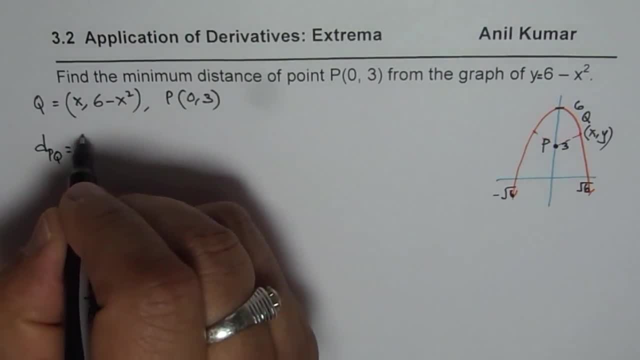 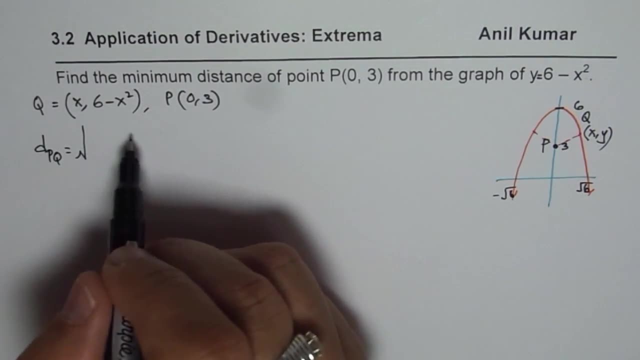 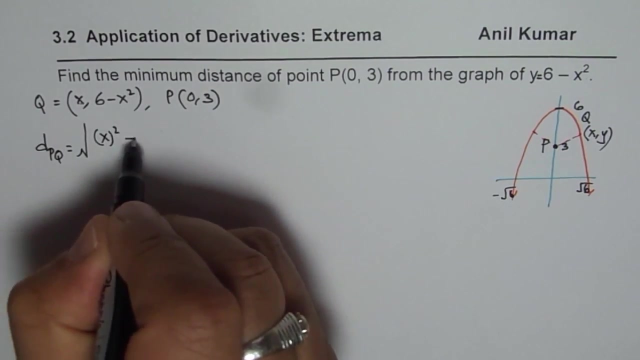 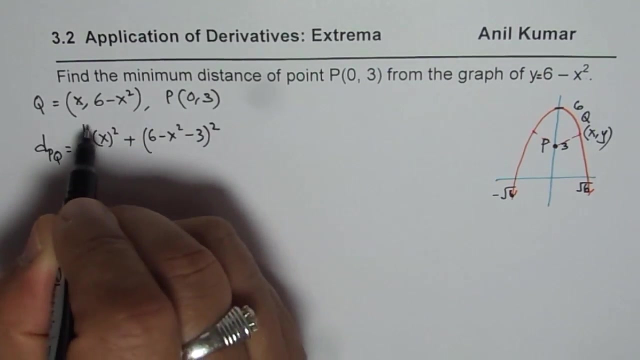 So distance between P and q will be square root of x2 minus x1 plus, I mean square of that plus y2 minus y1.. Let us use this as the second point. So we have x minus x2.. So that is 0, that is x squared plus. that is a y value: 6 minus x squared minus 3, right, Whole square. So that is my, so that is the distance. 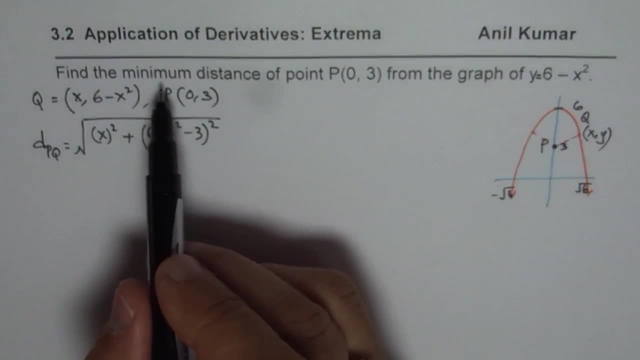 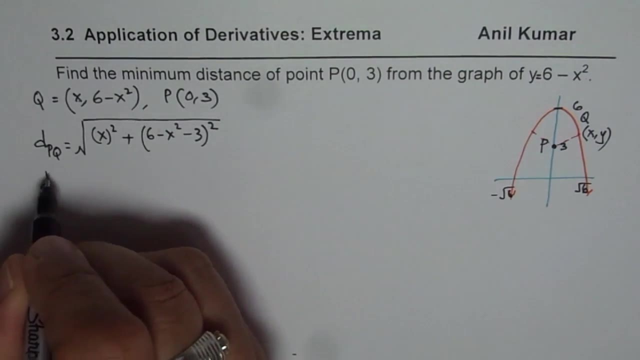 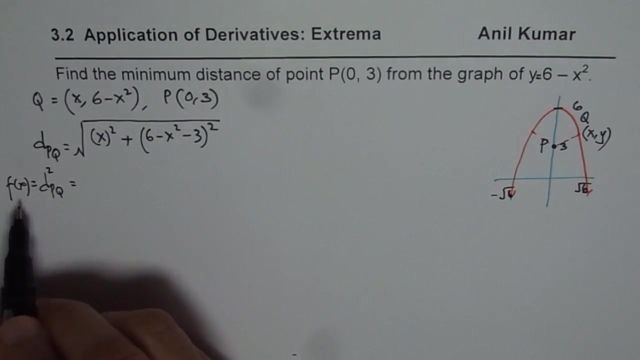 Now, since we need to minimize the distance, even distance square minimized will give you minimum distance right. So the idea is we could actually square both sides right And get new function. We call this as f of x And we'll minimize this. 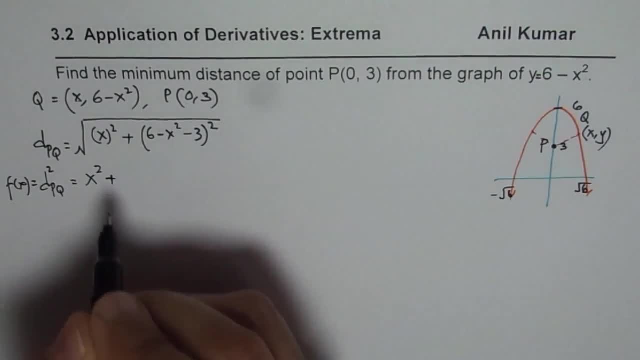 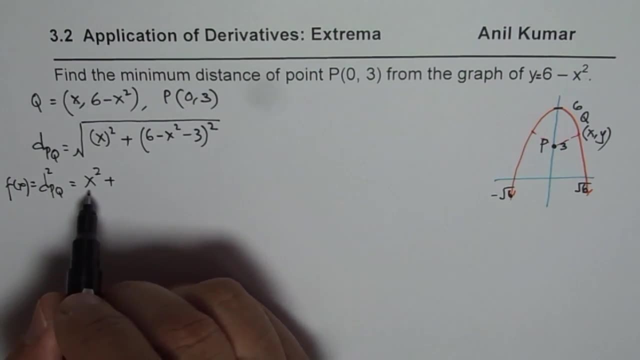 This particular function which gives us x squared plus. it helps in, you know, simplifying the calculations. I hope you appreciate the idea: Minimizing square of the distance, So we don't deal with a complicated derivative. Let us expand this part, which is: you can first simplify this. 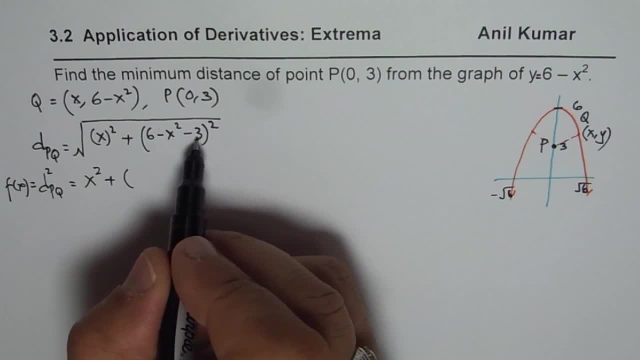 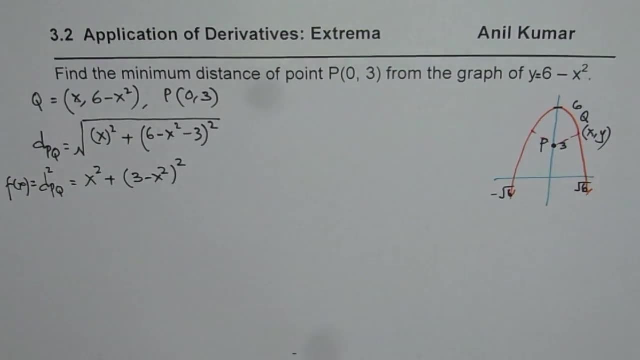 So it is 6 minus x squared minus 3.. So it could be written as 3 minus x squared right, So 3 minus x squared whole square. So that is what your second factor is. Now let us find derivative of this function. 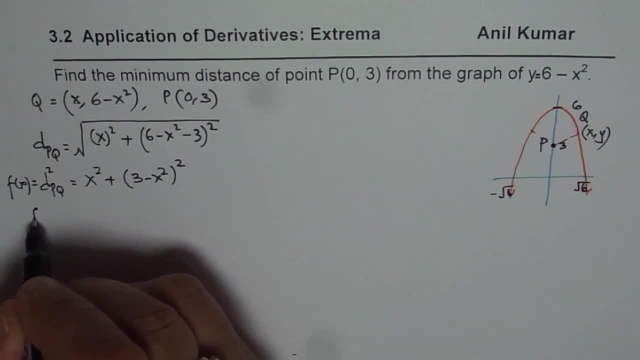 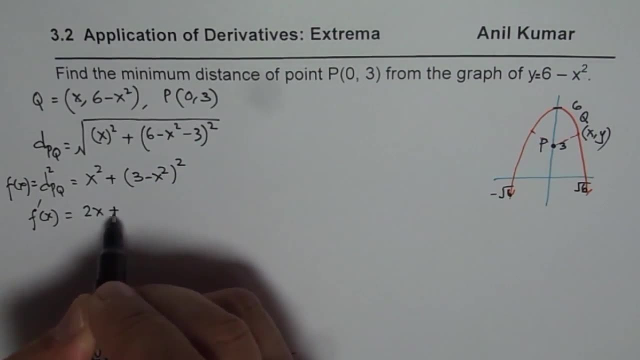 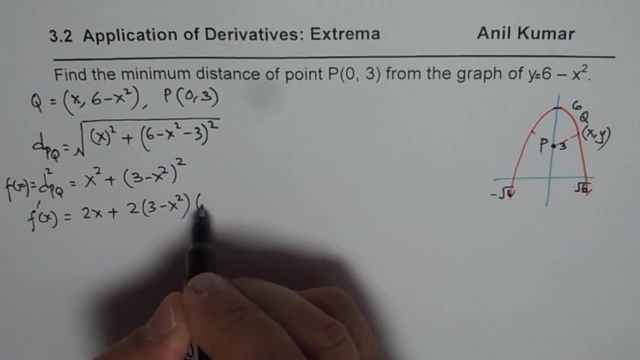 So minimum, we have to see a few things. That is, the derivative will give us the critical points. So let's find derivative of this. Derivative is 2 times x right Plus 2 times all this. That means 2 times 3 minus x squared times. derivative of inside function, which is minus 2x. 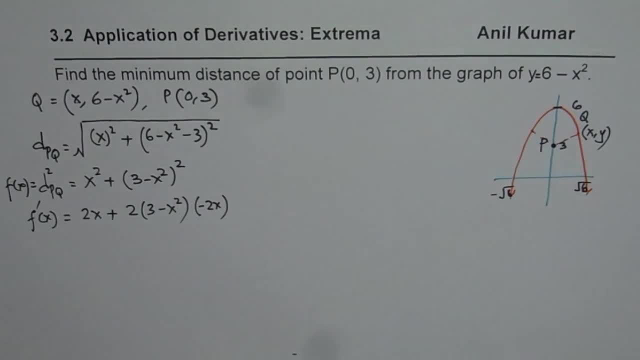 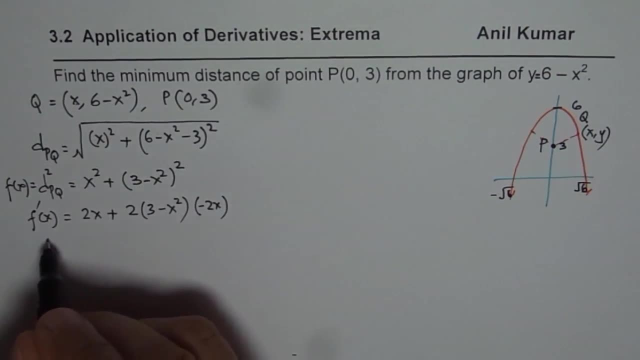 Is that okay? So that is the derivative. Next step is we need to find the minimum. So we'll find critical points. To find critical point, we'll equate derivative to 0, right, While it cannot be undefined, it is defined all throughout. 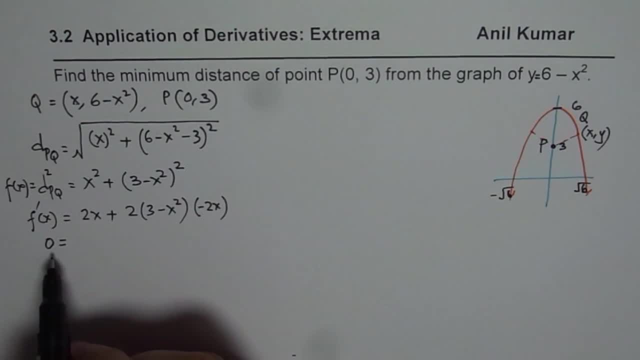 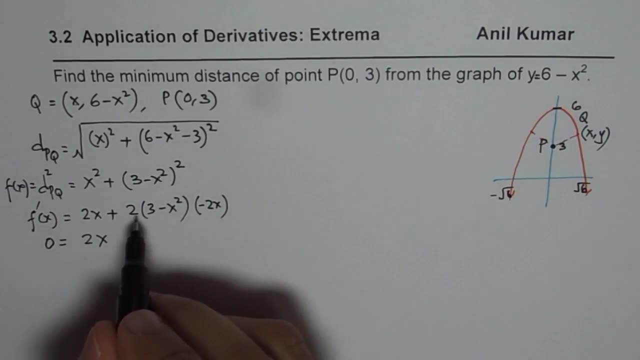 So the only possible value, critical value or number- will be when the derivative is 0. So let's equate to 0, solve the equation, So we have 2x, And here let's open this bracket. So minus 2 times minus 2 is minus 4.. 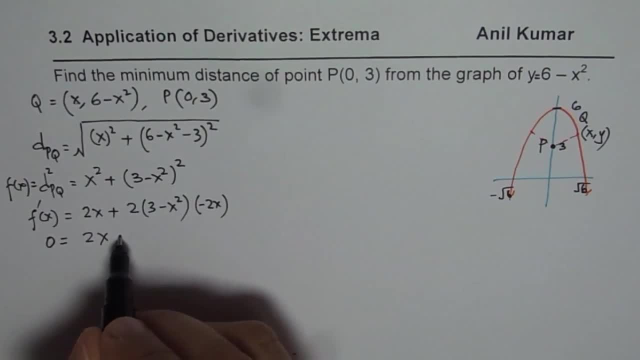 So we'll multiply. We'll multiply by minus 4, all the terms inside. So it gives us minus 12x, Minus, minus becomes plus And gives us 4x to the power of 3, right, So okay. 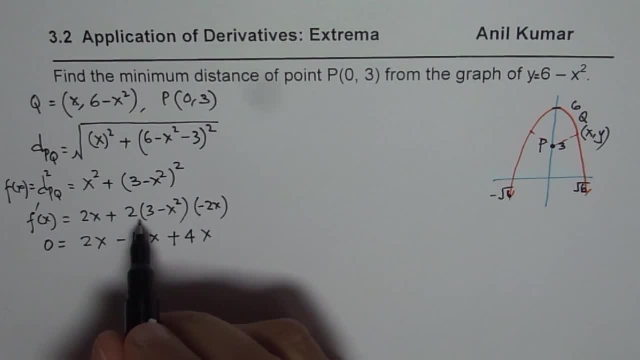 So x cubed. So okay, So this is minus minus 4x cubed. Okay, So that becomes Our equation. Now we can factor out 2.. So we get 0 equals 2. 2x. Let's rearrange and factor. 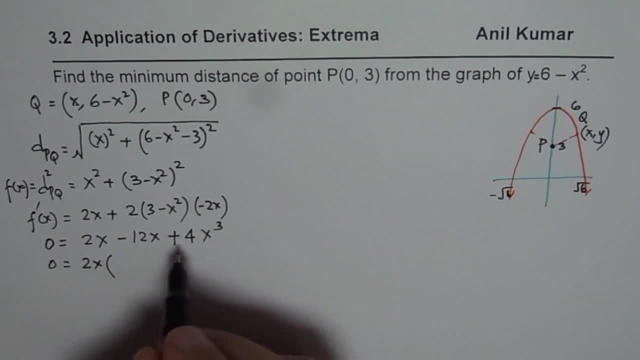 So 2x is common factor. So I'm writing this first now. So I get here. If I take out 2x, I get 2x squared, And 2x gives me 1.. We'll combine these two terms, right. 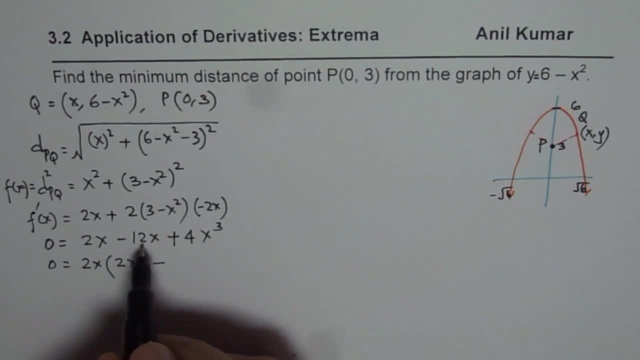 So that is minus 10.. So it gives me 5, right, So that gives me 5.. Okay, So I'll just combine these two: 2 minus 12 is minus 10.. So minus 10x, I'm taking 2.. 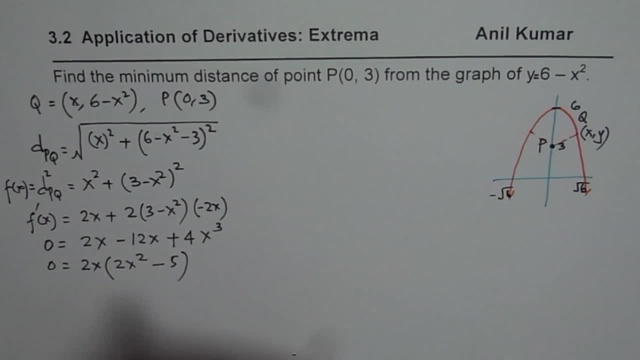 So I get minus 5.. That's fine. So that gives us solution. x could be equal to 0.. Or x is equal to, in this case, 5 over 2, square root With plus and minus, So we can write square root 2.5.. 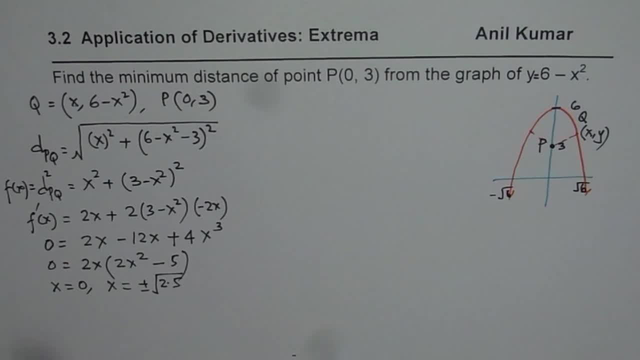 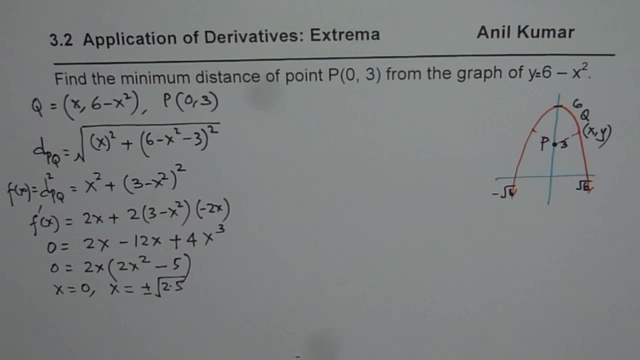 Is it okay? So that is. These are the possible solutions. So we get 3 critical points in our system. Now let's find out what is the distance for these 3 critical points, right? And then we'll see which one is the minimum distance, right? 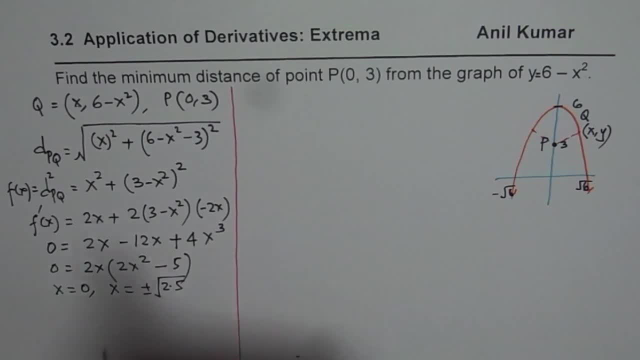 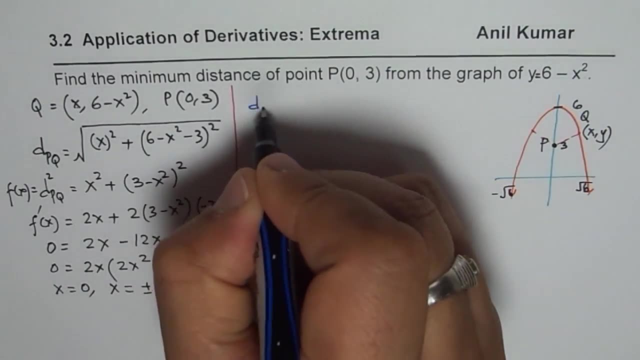 So we'll substitute these values in the equation itself to find which is the minimum distance, right? So distance dpq is equal to square root of x squared. If I write x equals to 0, then it will be 0, right? 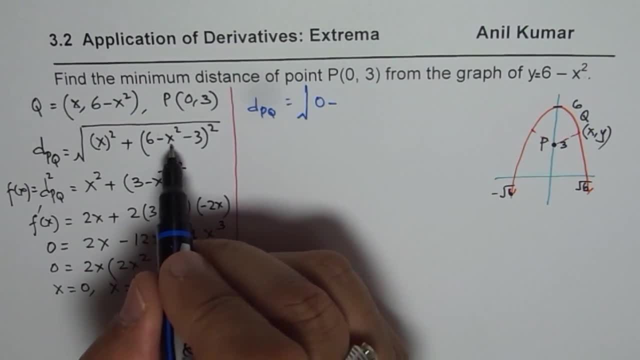 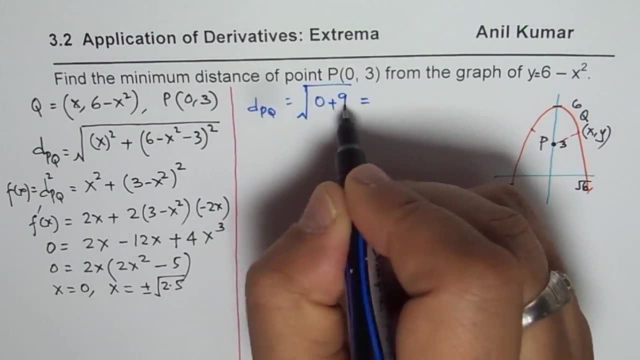 Minus 6, minus 3, x is 0.. So we have 6 minus 3, 3 squared is 9, right? So plus 9,, which is equal to 3.. So this is 3 units. 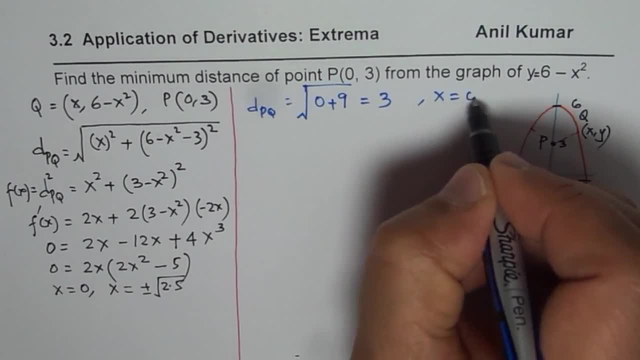 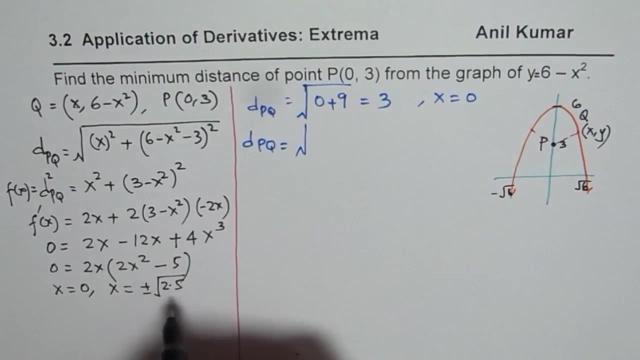 If I use 2.5, so this is for x equals to 0.. If I use 2.5 square root, then the distance dpq it will be equal to. We are substituting this square root 2.5 value here for x. 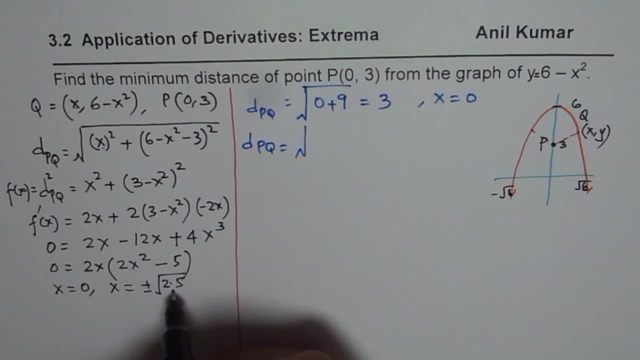 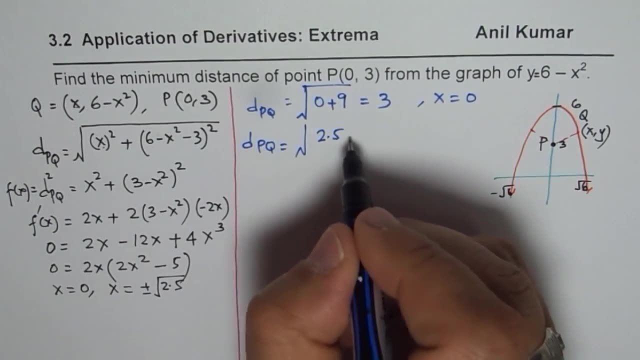 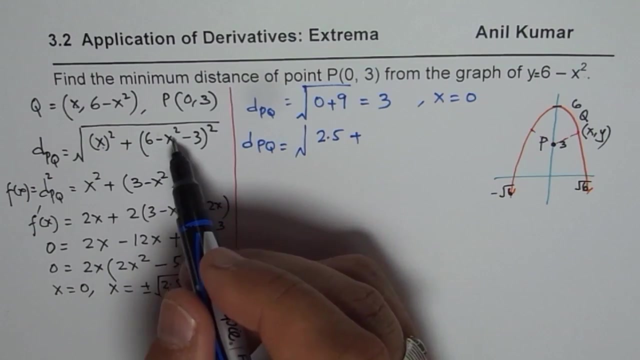 So that gives you square of 2.5.. Whether it is positive or negative will be positive. 2.5, right, So it is 2.5 plus. Now, if I write 2.5 square, so I got 2.5 here also. 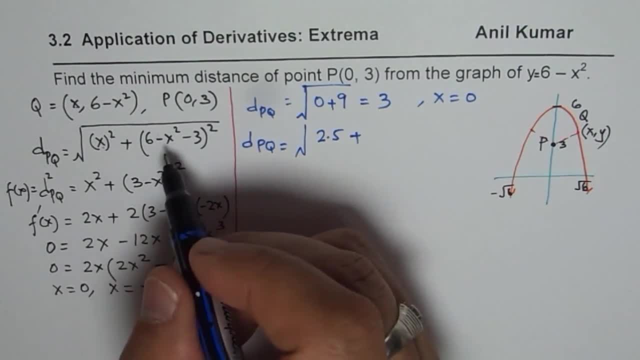 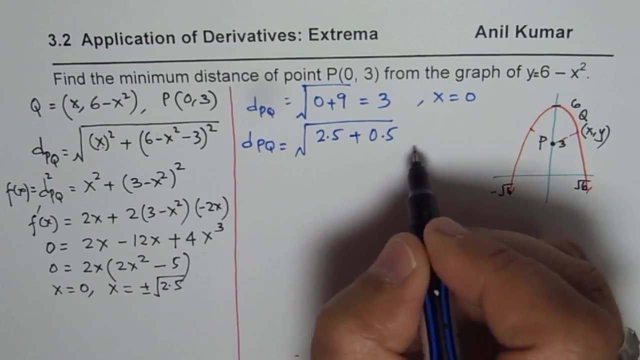 So 3 minus 2.5 will give me, because that is 3.. 3 minus 2.5 will be 0.5.. And this is for x. equals to plus or minus square root of 2.5.. Is it okay? 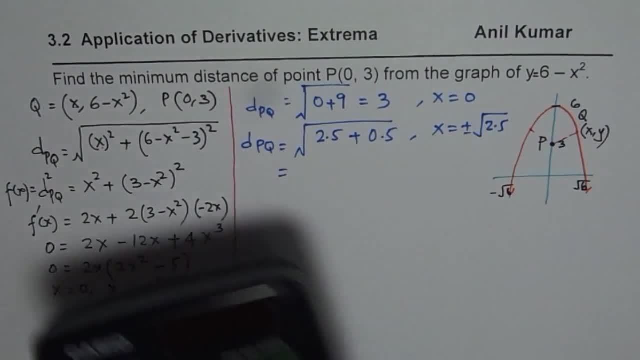 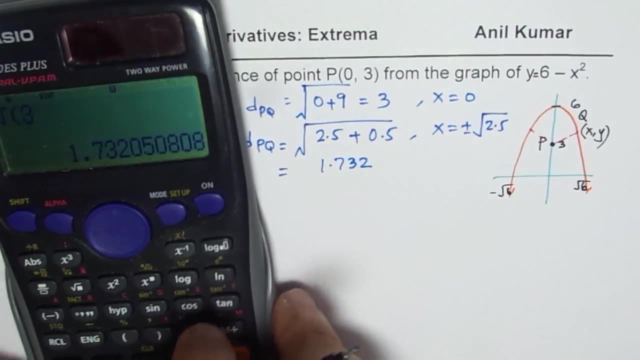 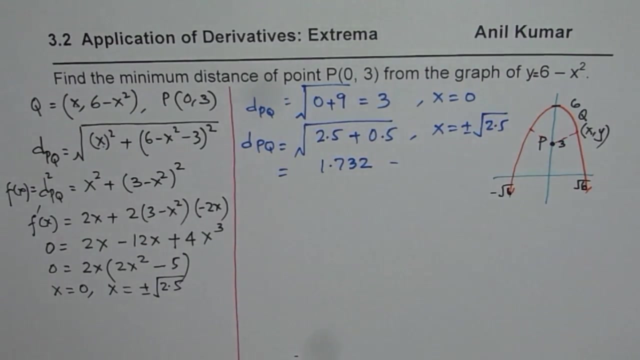 So that gives us a value which is approximately square root of 3, right, So square root of 3,, which is approximately 1.732, right. As you can very clearly see, this distance is minimum, right, So that gives you the minimum distance. 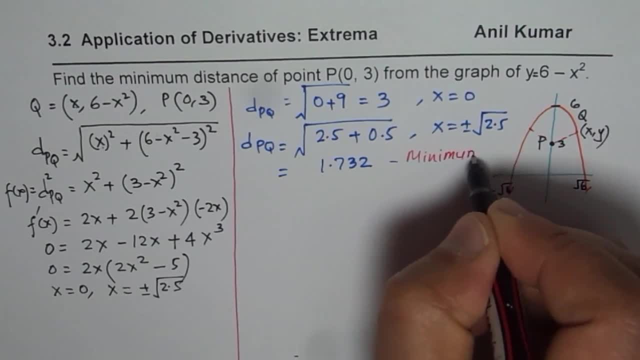 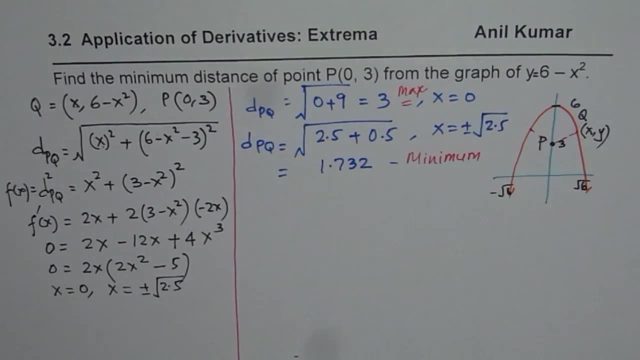 So this is your minimum distance And that will turn out to be the maximum distance, right? Okay, that is a different story. Those are the two critical points, Okay, So that is the minimum distance for the given graph And this is the process of doing it. 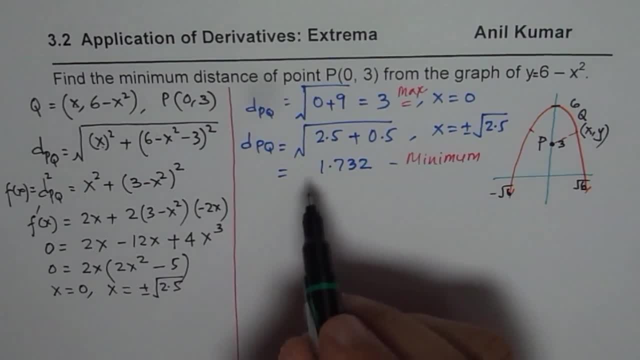 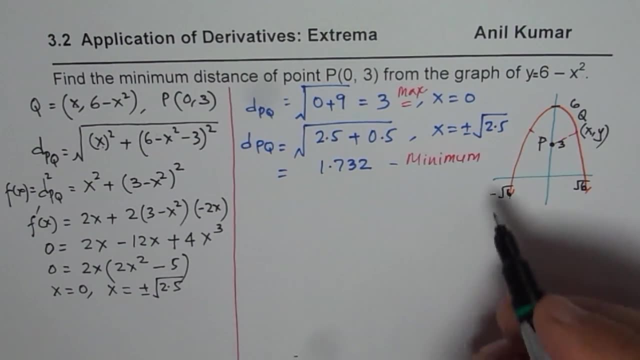 Now it is important to you know there are different ways of really checking whether this is minimum or not. One of the ways is to find the second derivative, And the other way is to analyze the derivative itself. So what you can do is you can analyze the derivative. 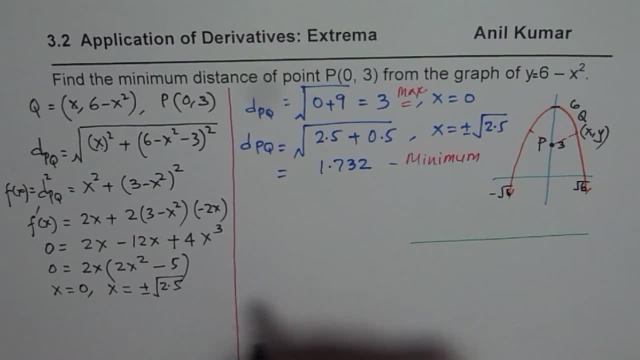 You have two particular values- 0 and 2.5, which is plus and minus. Rather, there are three right. So what you can do is let us say this is 0.. This is 2.5 square root positive. 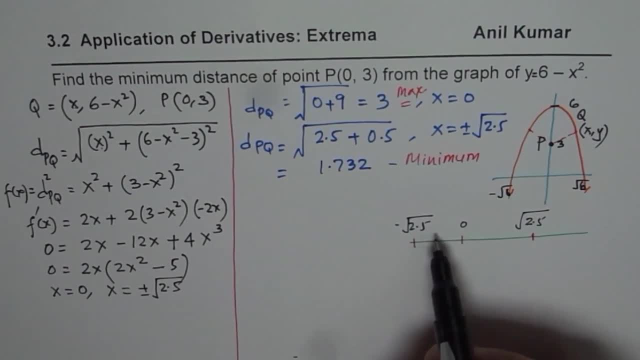 This is negative 2.5.. Now, in these cases, take a test point on each side right, So 1 could be a test point in each side right, Since square root 2 will be 1 point more than 1, correct. 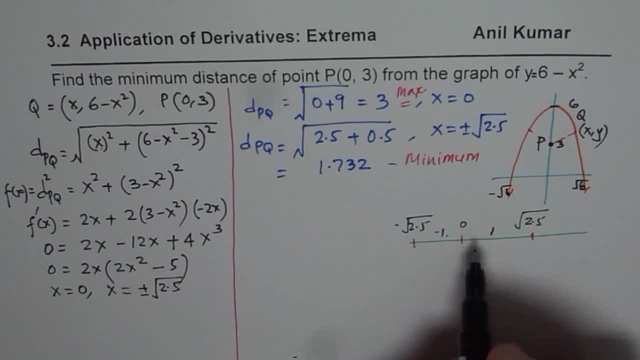 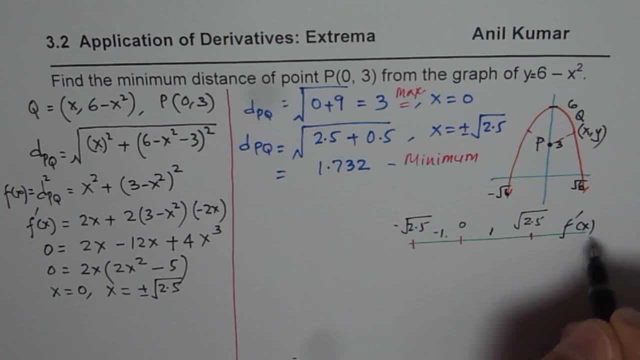 So plus or minus 1 could be good points to take. Okay, This is: we are analyzing the derivative for f dash x. We are analyzing the derivative for f dash x. That means the rate of change for f dash x at these points. 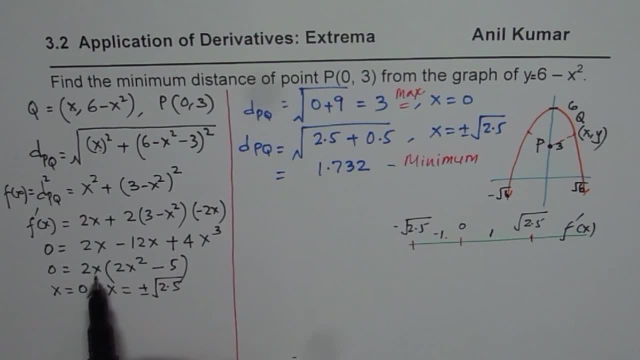 So if that was the equation, if I write 0, we get 0. So those are the critical points. If I write minus 1, which is on left side of 0. So if I write minus 1, this term becomes negative. 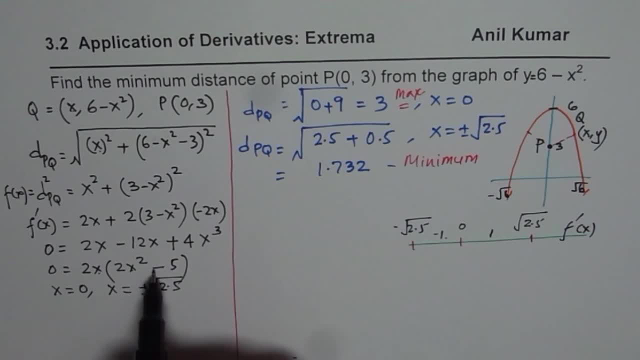 And here what we have is 2. Minus 5,, which is also negative, right. So this is negative for us. Minus 1, right Now, if I write 1, if I write 1 here, in that case this is positive. 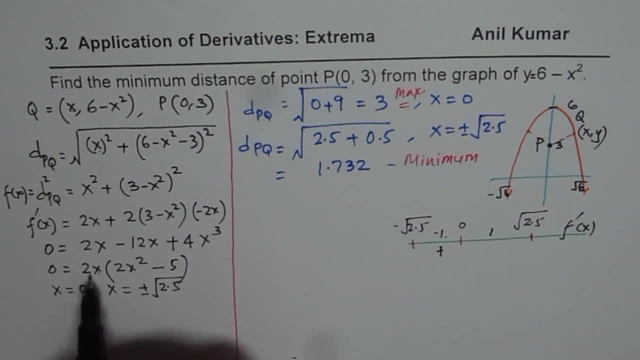 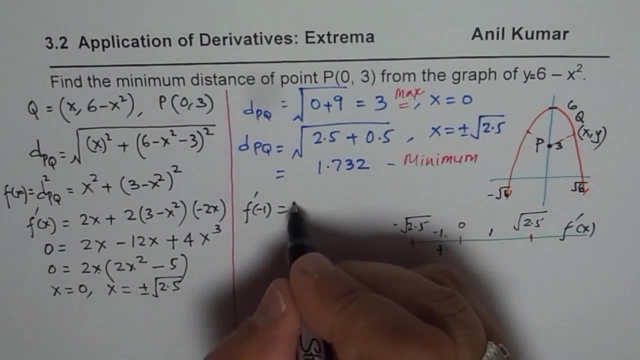 This is negative. Sorry, this is positive. I am sorry. If I write minus 1, that means to say f dash of minus 1 will be equals to let me substitute. So we have 2 times minus 1 times. 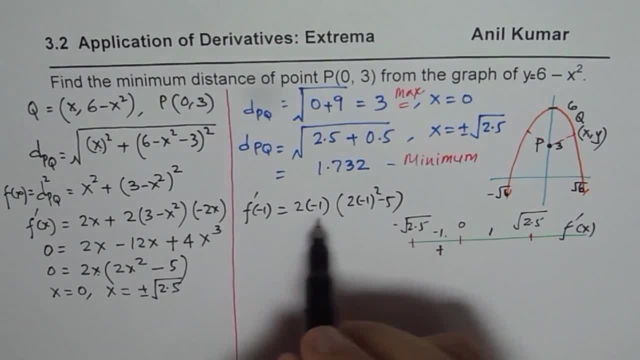 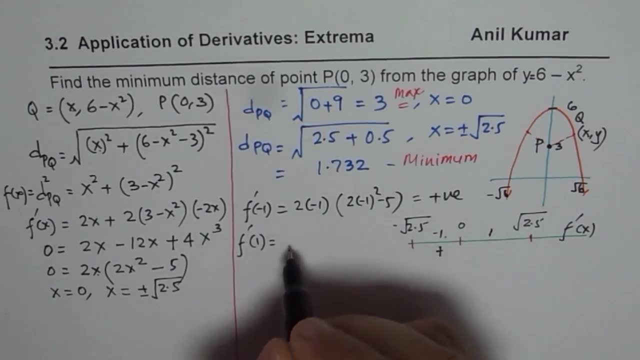 That will be 2 times minus 1, square minus 5.. So we get minus and minus. We get a positive value. Is that okay? If I write f dash at 1,, then this will be 2.. And this will be 2 minus 5, right. 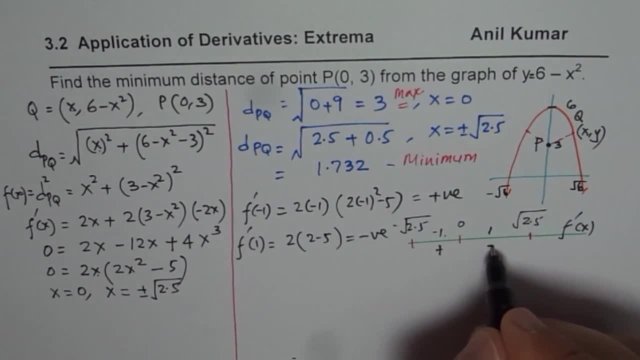 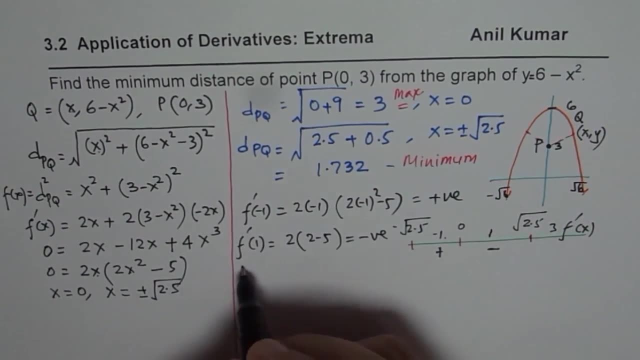 Which is negative, right, This is negative. We don't have to calculate the value, right? And if I take a value which is kind of, let us say 3 here, okay, So if I write 3 here, let us say f dash at 3.. 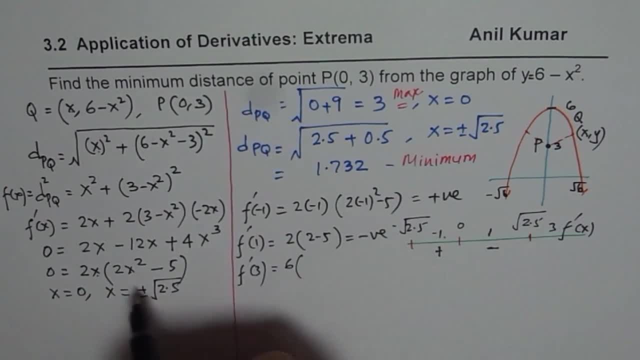 3 will be 6, will be positive here 6. And 3 square, so 9 times 2, 18 minus 5, which is positive right. So that really shows that the graph is positive on this side.